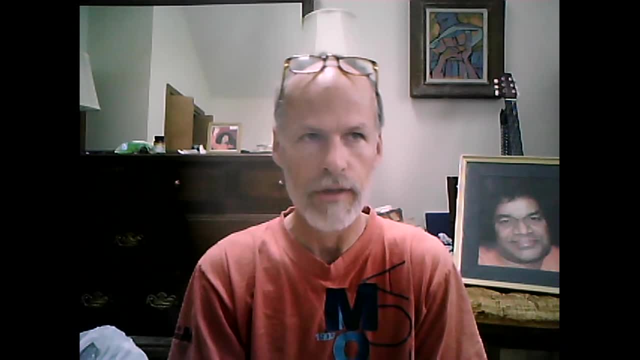 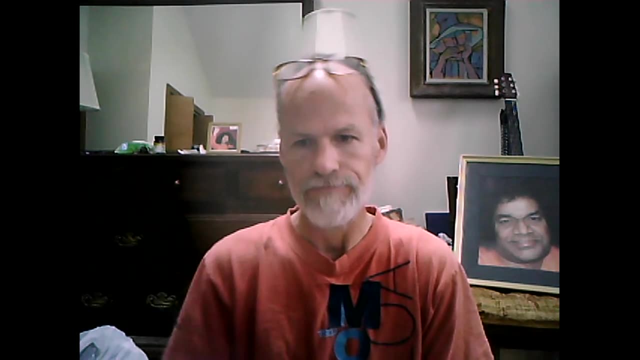 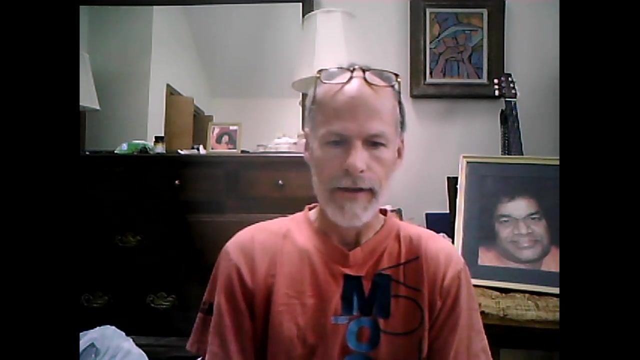 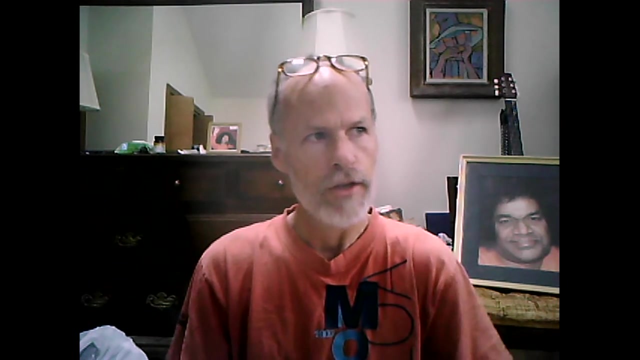 It's the kind of stuff you would have seen in Lear Keefe's book, where she used to be a vegan and then she gave up being vegan. She has some reasons, which are debatable, for why she did that. Some of the arguments that these folks make are like: when you have a grain-growing farm. 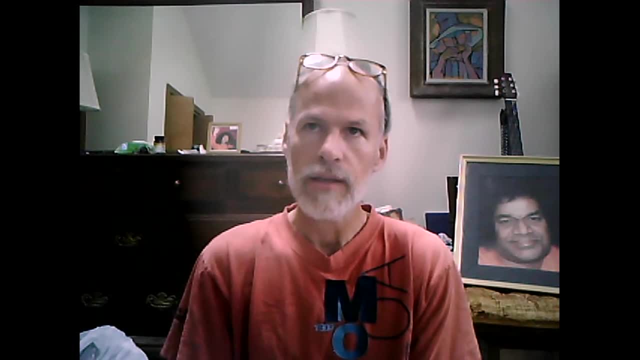 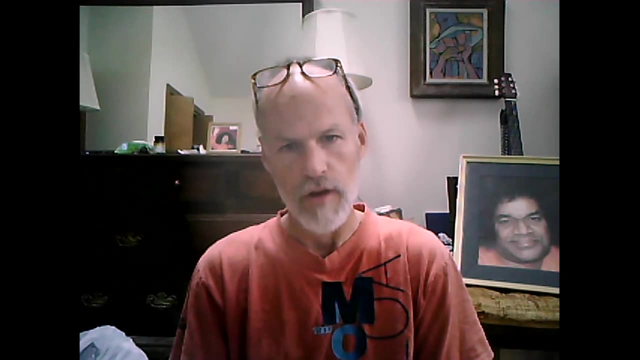 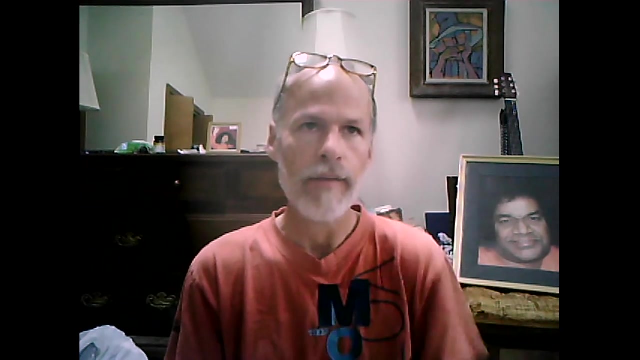 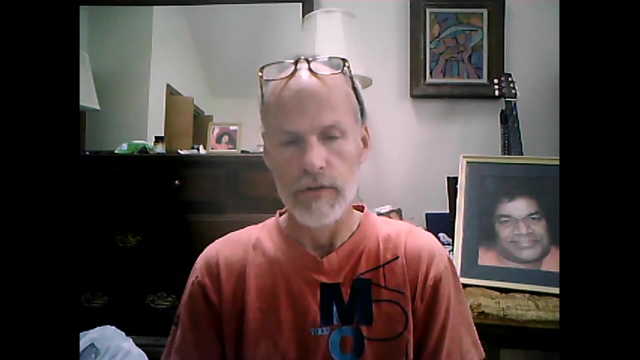 when you produce that grain. there could be little animals that live in the grasses which are killed when the grain is harvested, so like mice or birds or things like that. Another argument is the growing of bananas is an ecological nightmare and therefore we should be more concerned with banana production than with cattle production. 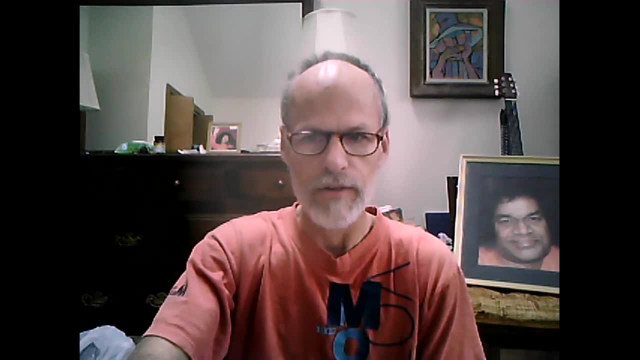 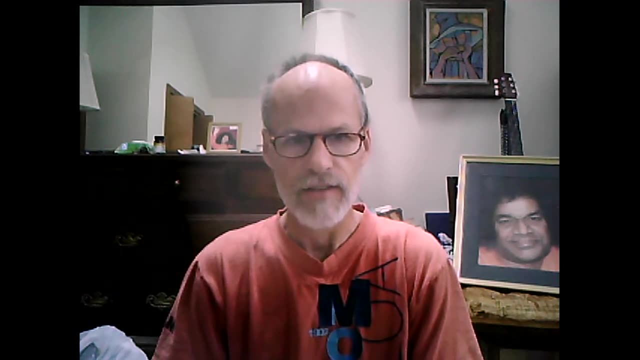 Well, while there's truth to the fact that industrial agriculture, like banana production, is not ideal, it's not anywhere near comparable to the damage caused by animal production for animal foods, And the same is true with this. you know, yes, there's probably small animals in some of the grain produced. 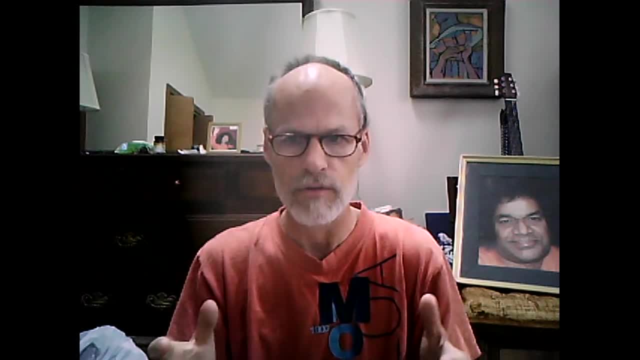 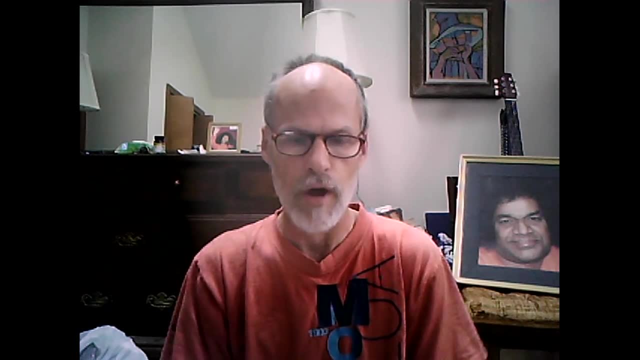 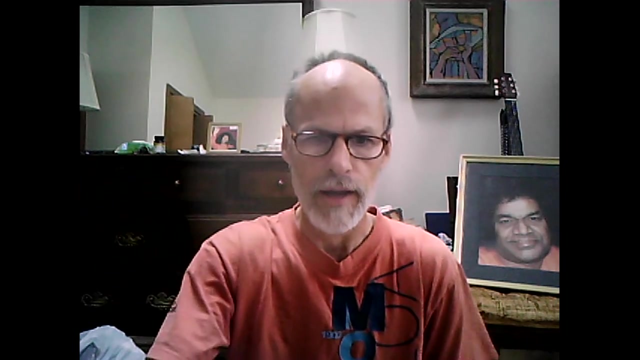 but it's nothing, it doesn't do anything, it's not comparable in terms of, you know, environmental damage and then also health and ethics of you know, broad-based, large-scale animal harvesting, like cattle. So, you know, I pulled up a little bit of data on this. 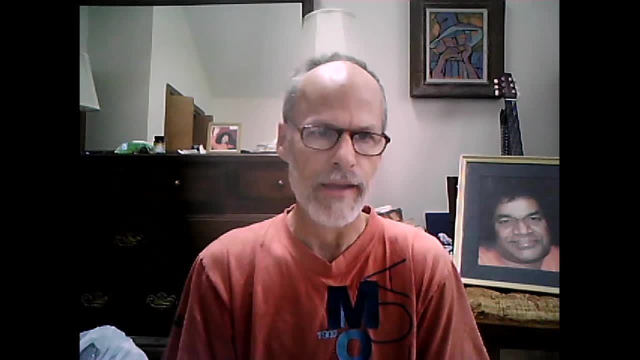 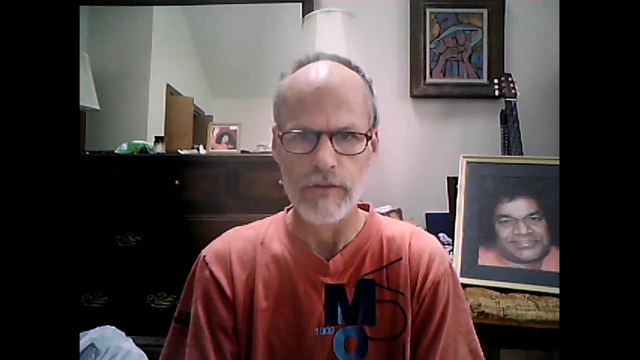 Here's a pie chart showing causes of deforestation in the Brazilian Amazon from 2000 to 2005.. So you know, this is a pie chart showing causes of deforestation in the Brazilian Amazon from 2000 to 2005.. 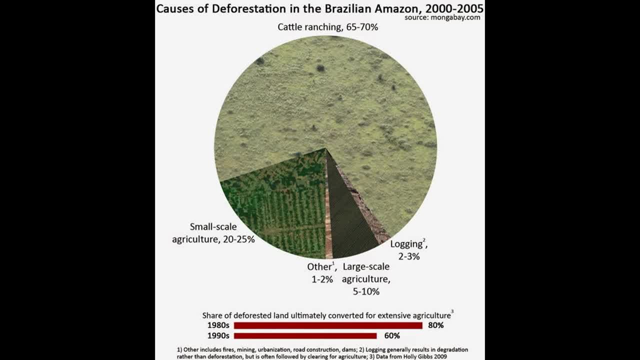 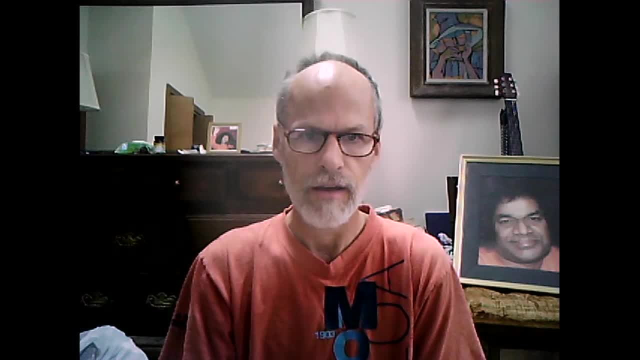 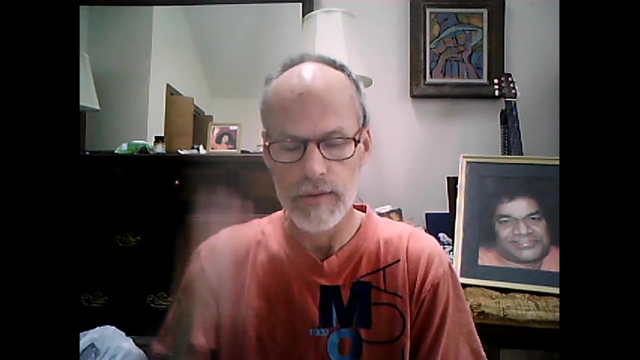 So cattle ranching took up 65% to 70% of the deforestation in the Brazilian Amazon. Small-scale agriculture took up 20% to 25%. Large-scale agriculture- which would be like bananas or you know, other large-scale crops- 5% to 10%. Then they had logging 2 to 3 percent, Other 1 to 2 percent. In other words, cattle ranching 65 to 70 percent. Large-scale agriculture, like the kind criticized by paleo-enthusiasts, 5 to 10 percent. So should we really be as worried about bananas as we should about cattle? Cattle ranching takes up 65 to 70 percent of the deforestation in the Brazilian Amazon. Large-scale agriculture 5 to 10 percent. I'm not saying all large-scale agricultural practices are pristine and to be glorified. They probably should be looked into and improved to the degree possible. 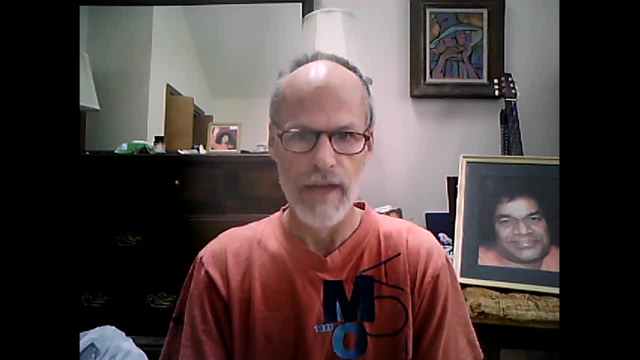 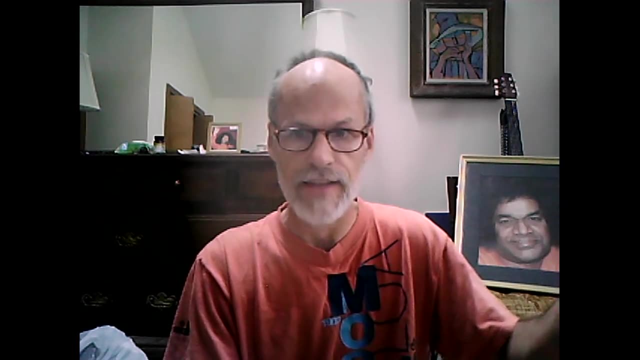 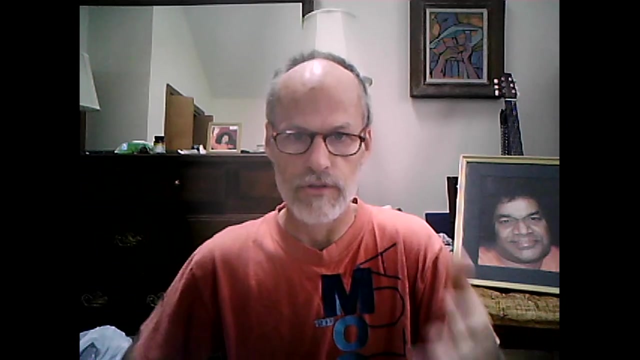 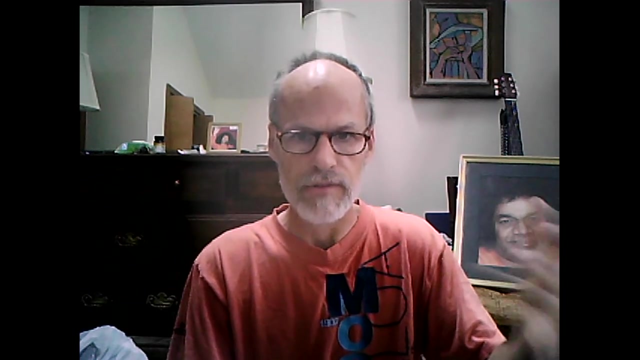 But you know we're not… We're not going to stop large-scale agriculture. We have to feed the planet. I mean, if everybody starts growing enough food in their backyard that we can stop large-scale agriculture, fantastic. I don't see that happening. But to suggest that large-scale agriculture is the real problem and not cattle ranching or the insane demand for animal products and people's diets, that is the problem. 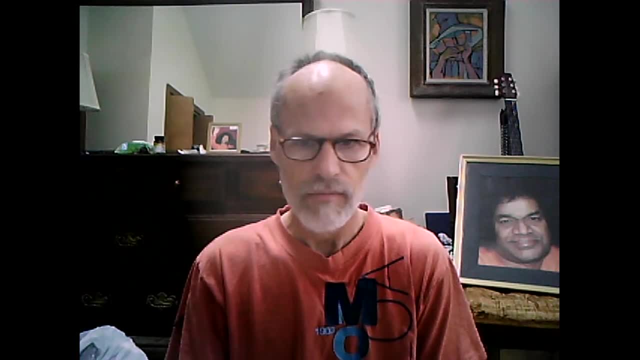 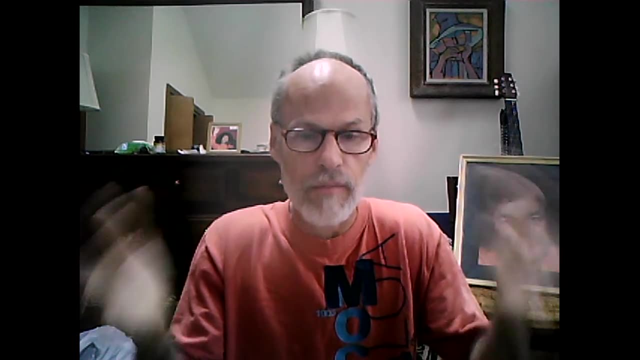 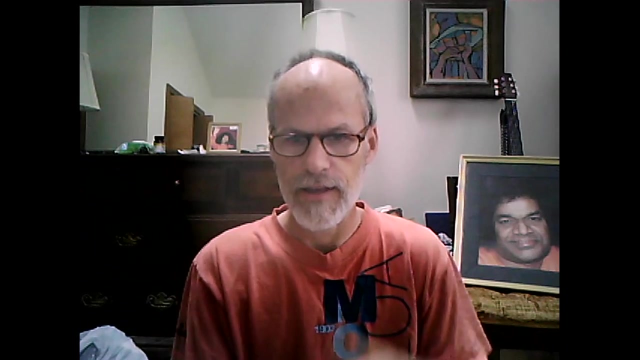 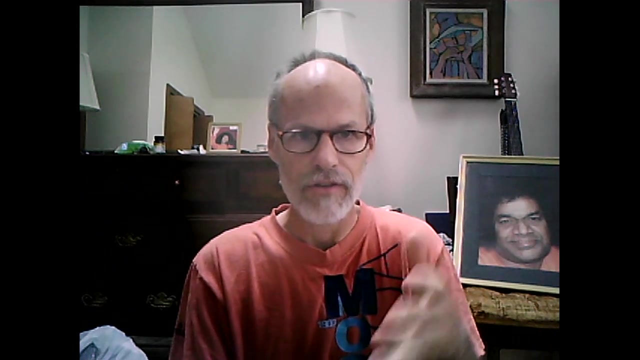 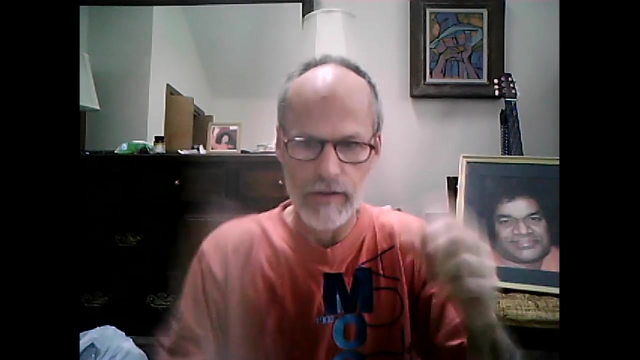 And often these paleo-arguments… They only address one issue and they don't even address that accurately. It's a misguiding, misleading form of… It's a misdirection, you know, And it's a false dichotomy. It's just absurd to compare the production of bananas to the deforestation caused by the raising of cattle. It's like you're comparing something tiny to something huge. 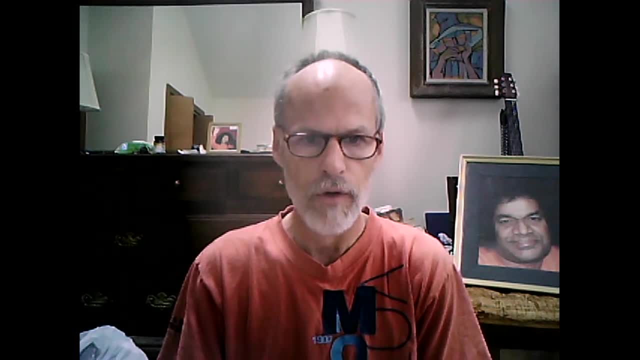 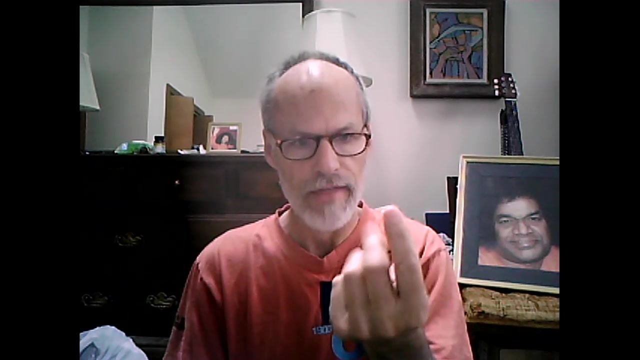 It's a huge misdirection. So you know, be honest, Be intellectually honest when you're making these comments, And if you're going to try and justify meat-eating, you're going to have to address all three aspects of animal ethics: health to the individual and the environmental damage. 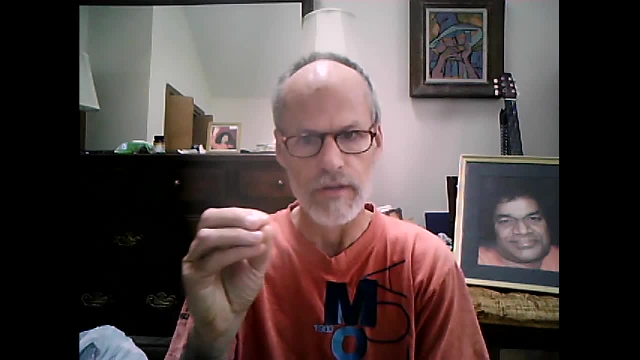 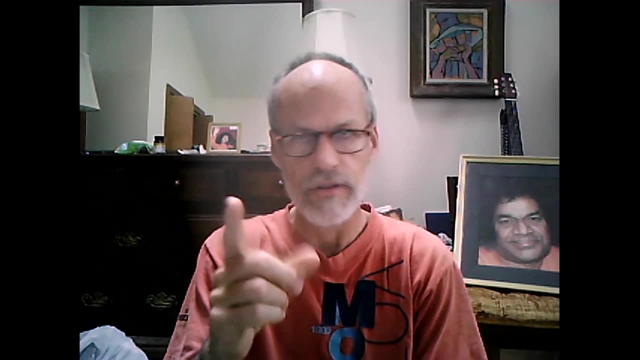 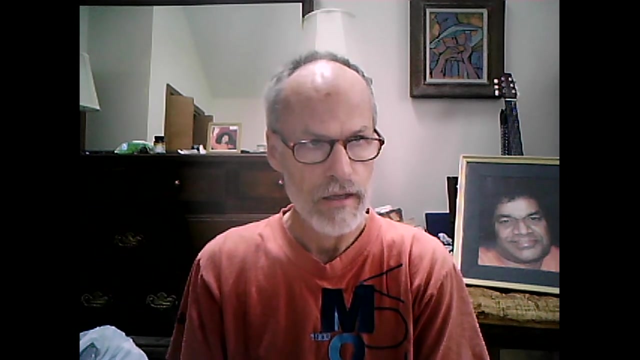 All three of these have to be addressed. So oftentimes, with these you know, animal-eating proponents… They only address one. They're usually saying something like: well, it's not that environmentally damaging. And then there's this thing of you know, we need cattle to have the right kind of soil. 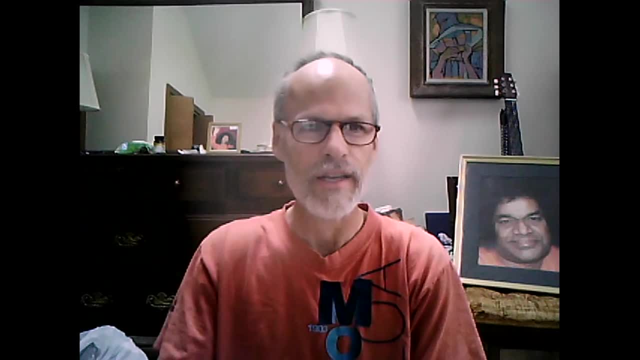 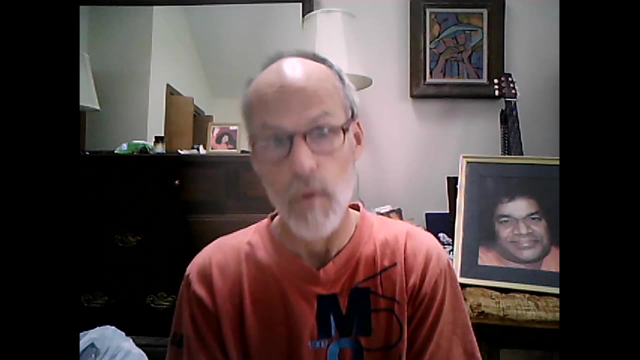 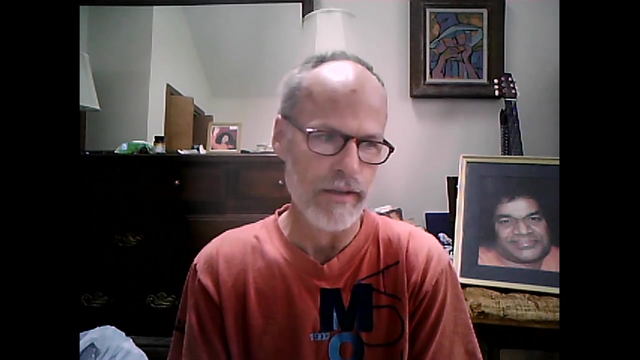 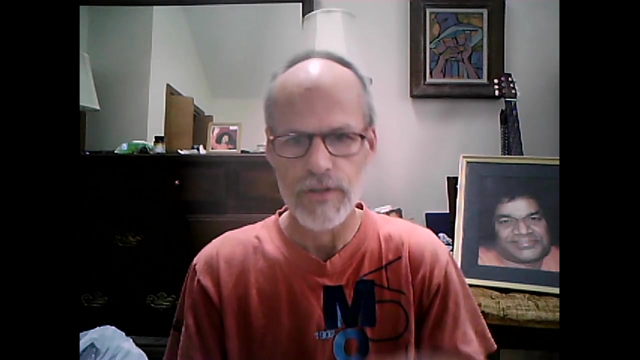 You know this is totally inaccurate. I was just reading the other day about grass-fed beef and how it causes more CO2, more methane, than beef that's grown…. …in enclosed spaces. So it's more environmentally damaging due to the fact that cattle who are grass-fed need more water and they produce more methane. 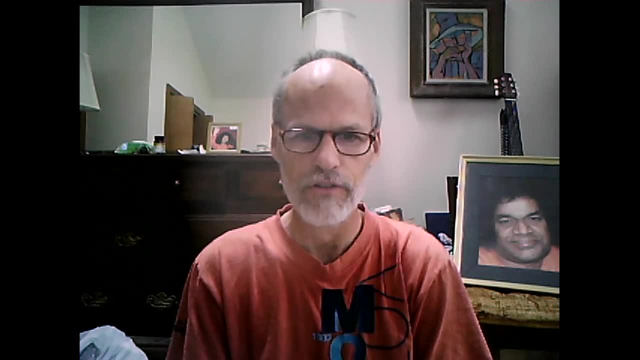 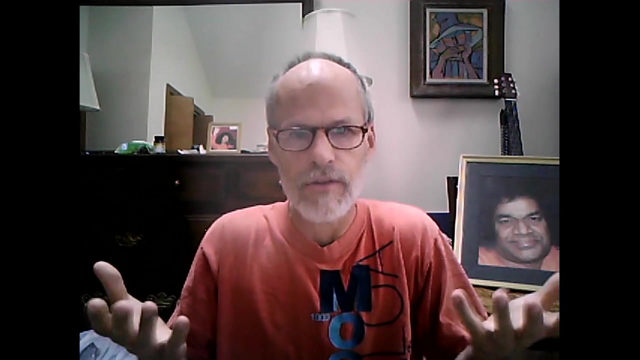 So you know, these are just…they're just shallow arguments that if you just look under the surface they have no merit. So get your facts straight. paleo folks, and really you know, try to present a full… …complete argument, and you can't, You can't. These things are undeniable. The amounts of water consumed for cattle ranching are astronomical And as we have this drought occurring in California, soon to be occurring elsewhere, you know who knows how much it's already occurring in third-world countries, in the Middle East, that sort of thing.